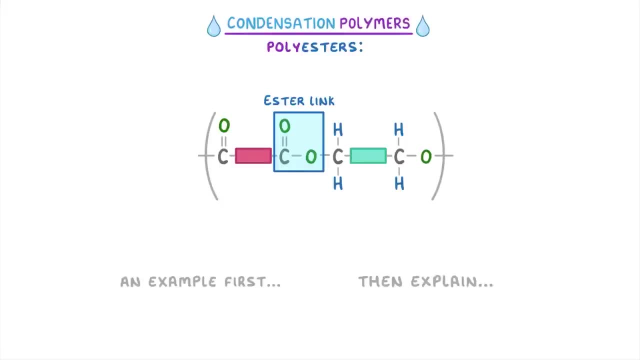 exactly what's going on afterwards. Like all polymers, condensation polymers are made up of lots of individual monomers. With polyesters, though, a common combination is to use two different monomers: A dicarboxylic acid monomer which contains 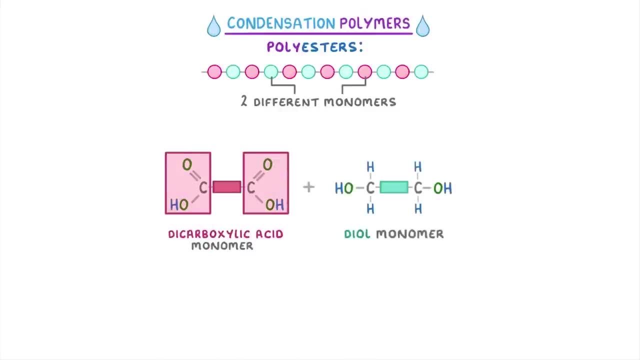 two carboxylic acid groups and a diol monomer which contains two alcohol groups. And as a quick aside, if you haven't seen these colored rectangles within molecules before, they just represent the rest of the molecule and we tend to use them in general. examples like here: 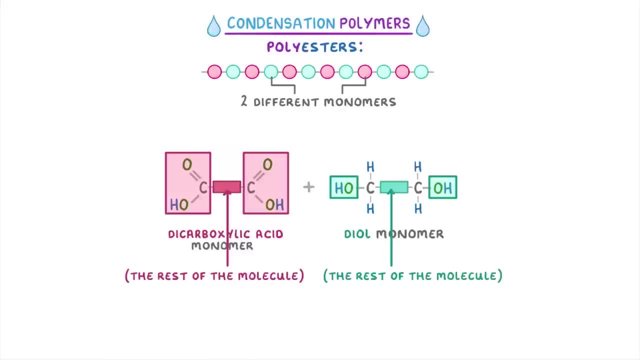 where we don't want to make things complicated by showing the specific molecules. In order for the two monomers to combine, the dicarboxylic acid has to give up its OH group and a diol gives up a hydrogen atom which contains a diol monomer which contains a diol monomer which contains a. 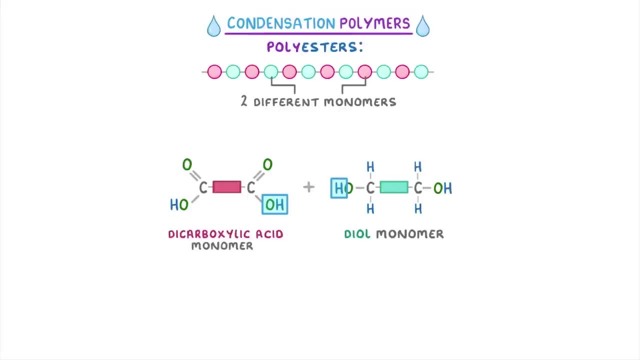 hydrogen atom from its OH group, And when these three atoms combine they form a water molecule. This leaves this carbon from the dicarboxylic acid to bond directly to this oxygen from the diol, And it's this bond that we call the ester link. 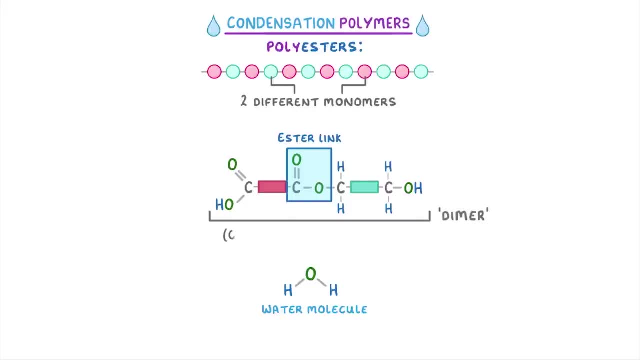 At the moment this is technically just a dimer, because it's only two monomers combined. To show it as a repeating unit, though, we need to remove this OH and H from the ends and then point the empty bonds out to the sides so that they can bond on to other repeating units. And, importantly, 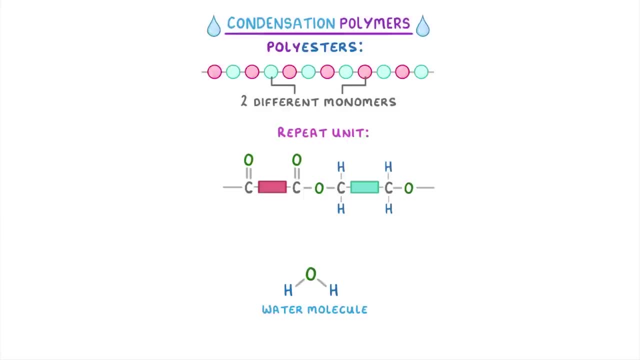 because we removed an OH and hydrogen again, it will form another water molecule. Then, to finish, we add these big brackets to either end that cut through the bonds. If we now put all of this together, we effectively had a dicarboxylic acid monomer plus a diol monomer. 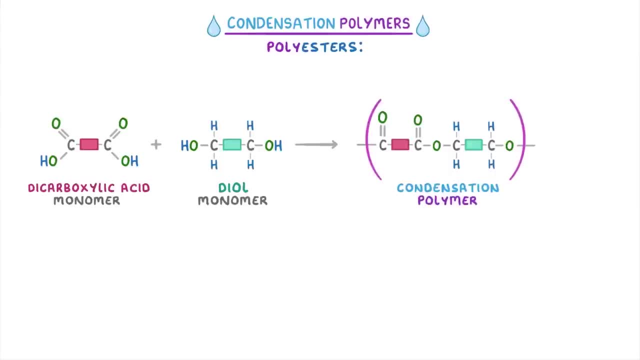 go to form a condensation polymer, Which in this case was a polyester, because this group in the middle is an ester link, And we also formed two molecules of water. In real life, this process often happens with hundreds or thousands of monomers, And so, instead of writing the exact number of molecules we have,